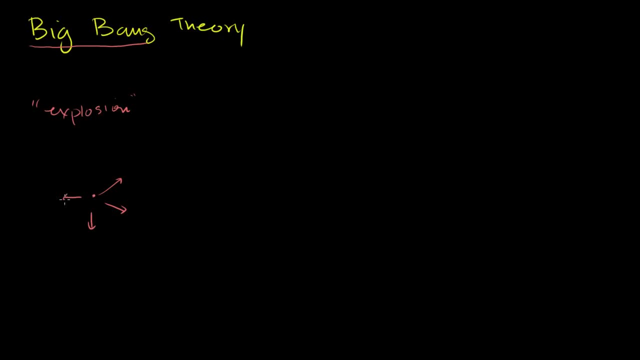 and then it exploded, And then it exploded outward And then, as all of the matter exploded outward, it started to condense, And then you have these little galaxies and super clusters of galaxies and they started to condense And then within them, planets condensed. 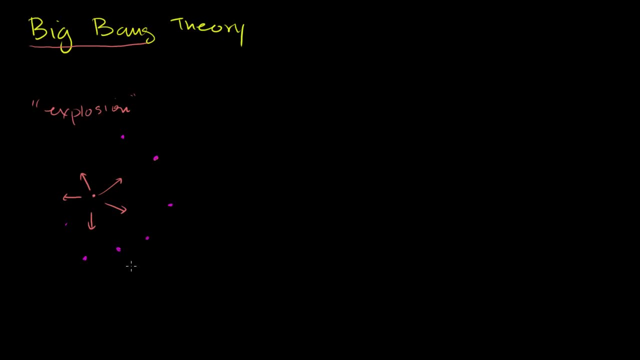 and stars condensed And then we have the type of universe that we have right now. But this model for visualizing the Big Bang has a couple of problems. One is when we talk about the Big Bang, we're not talking about the matter, just the mass. 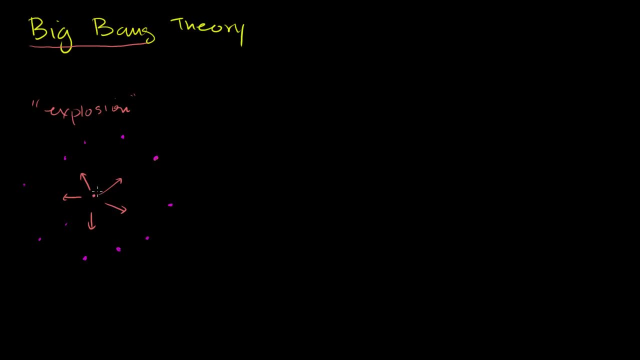 or just the matter in the universe being in one point. We're talking about actual space expanding. So we're not just talking about something inside of space like the physical mass, the physical matter expanding, We're talking about space itself. And so when you have this type of model, 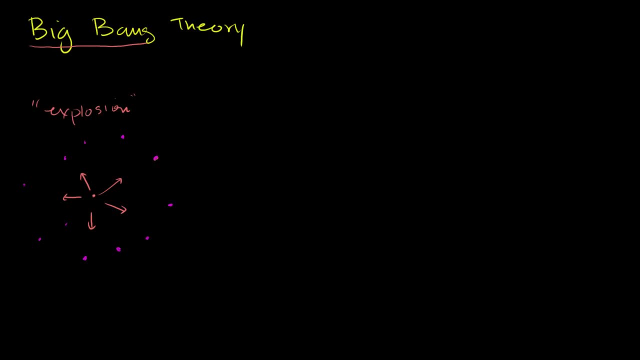 you have all of this stuff expanding, but you're like, well, look, isn't it expanding into something else? Maybe if the furthest out parts of this matter is right over here, what's this stuff over here? And so you say, well, wouldn't that be space? 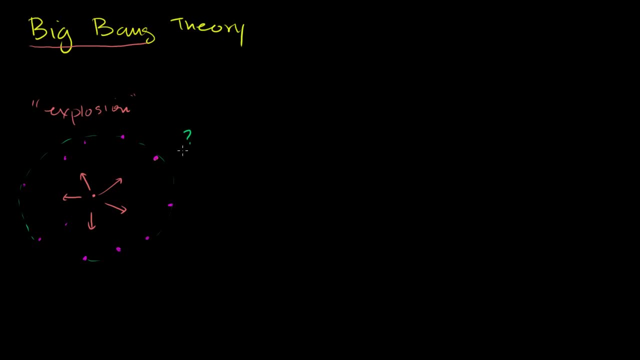 So how can you say space itself is expanding? And another idea that a Big Bang also implies is: if this is the furthest stuff out there, would this be the edge of the universe? Does the universe have space? Does it have an edge? 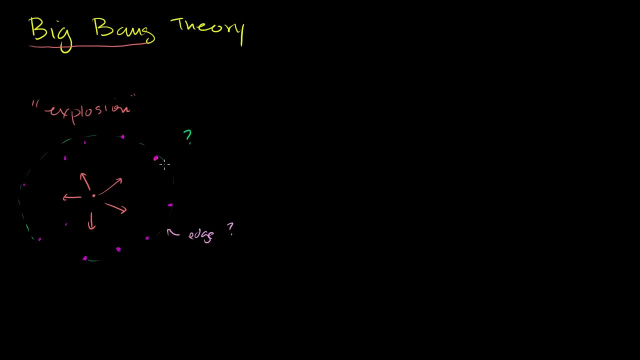 And the answer to either of those questions- and that's what we're going to try to tackle in this- is that, one, the universe does not have an edge And two, there is no outside space. We are not expanding into another space. 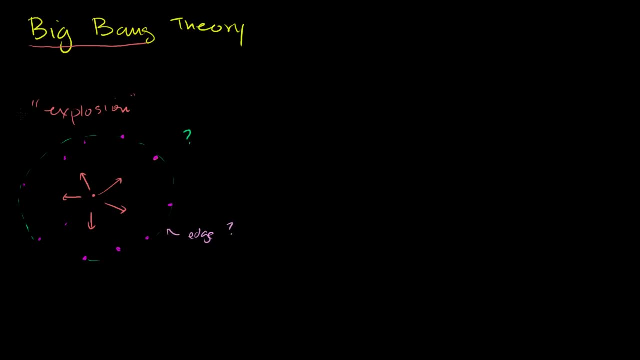 And I'm going to explain that. Hopefully, we'll see why that is the case right now. So the best way to view it- and we're going to view it by analogy- if I were to tell you that I have a two-dimensional space- 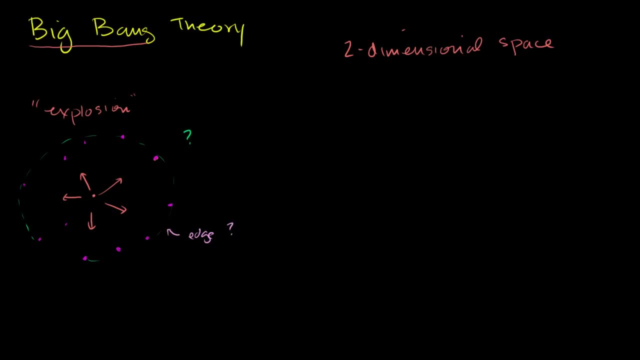 a two-dimensional space that has a finite area, so it's not infinite and it also has no edge. This once again, when you first look at it, seems difficult. How do I construct something that has a finite area but still has no edge? 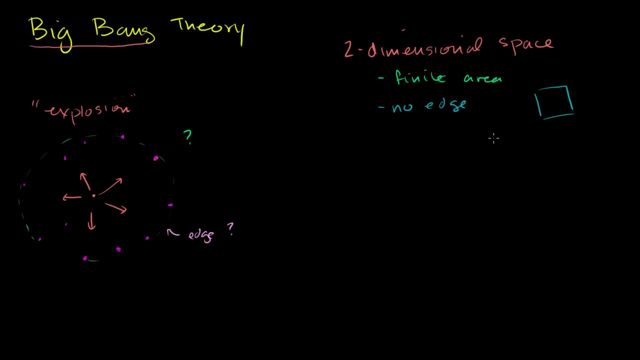 Every time I try to draw an area, it looks like I have to have some edges, And then you might remember What. What if that two-dimensional space is curved? What happens? And I think the easiest example of that is the surface of a sphere. 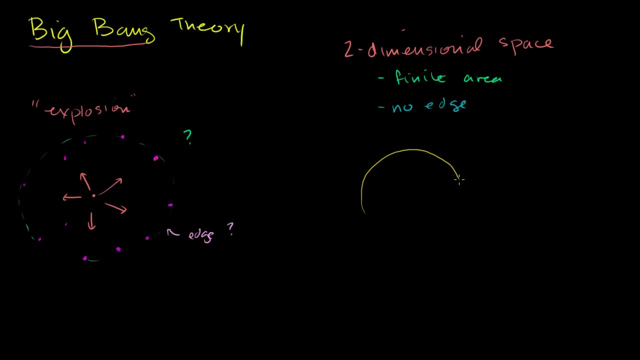 The surface of a sphere. let me draw a sphere over here. So this right here is a sphere. Let me draw some longitude and latitudinal lines on this sphere, On this sphere, all of a sudden, and I'll shade it in a little. 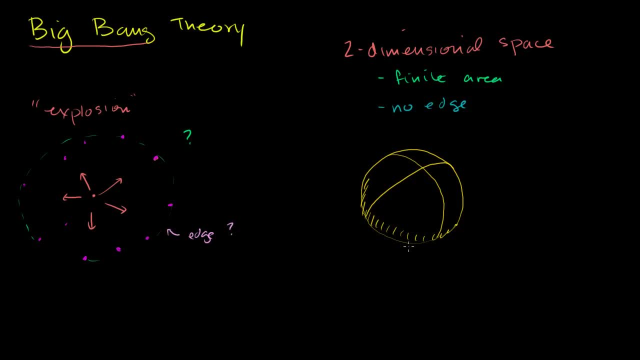 bit make it look nice. This type of a sphere. you have a finite area. You could imagine the surface Of a sphere Of a balloon, Or the surface of a bubble, Or the surface of the Earth. You have a finite area, but you have no edge. 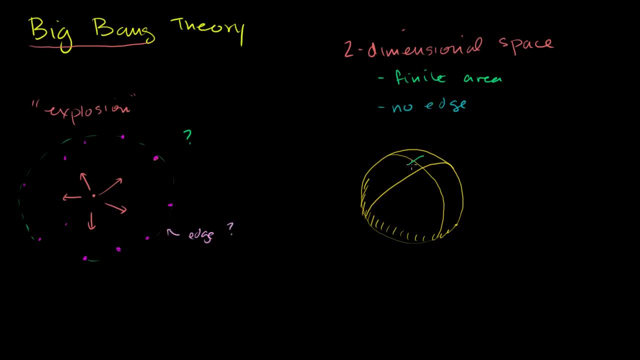 If you keep going forever in one direction, you're just going to keep going all the way around and come back to the other side. Now to imagine a three-dimensional space that has these same properties: a finite area and- and I don't want to say finite area anymore- 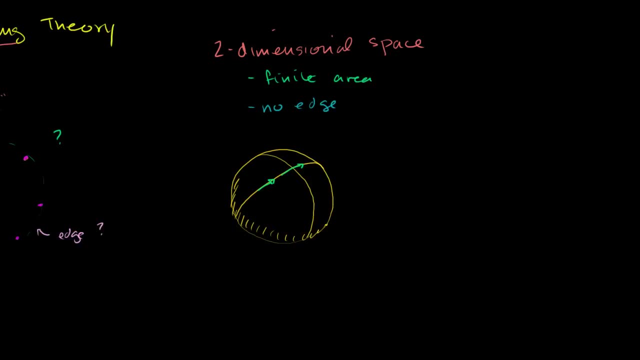 because we're not talking about a three-dimensional space. Let me draw it over here. So let's think about a three-dimensional space, So three-dimensional space Instead of area, since we're in three dimensions now. I want to talk about a finite volume. 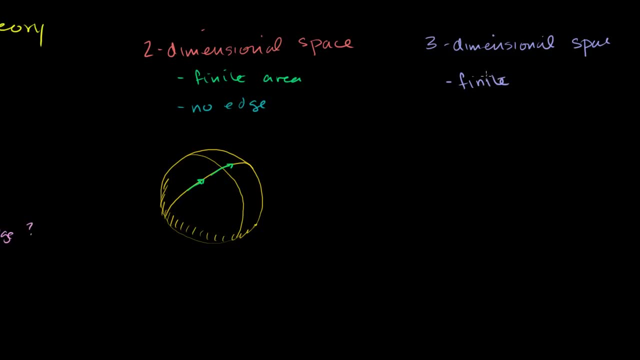 Finite volume And no edge. How do I do that? And when you think about it superficially, well look, If I have a finite volume, maybe it'll be in connection. It'll be contained in some type of a cube. 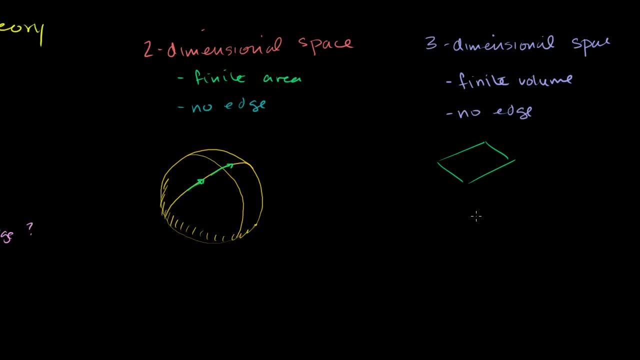 And then we clearly have edges in those situations. Or you could even think about a finite volume as being the inside of a sphere And that clearly has an edge- this entire surface over there. So how do you construct a three-dimensional space that has finite volume and no edge? 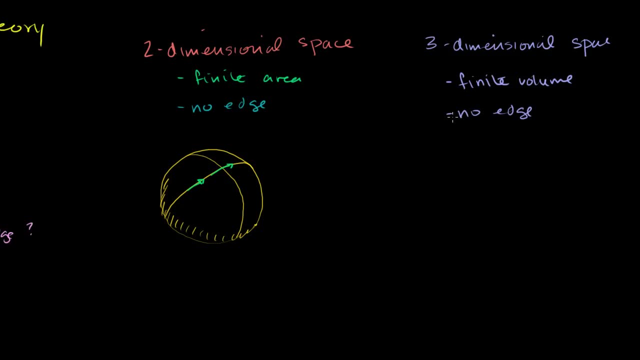 And that I'm going to tell you. right now, it's very hard for us to visualize it, But in order to visualize it, I'm essentially going to draw the same thing as I drew right here: What you have to imagine, and you almost. 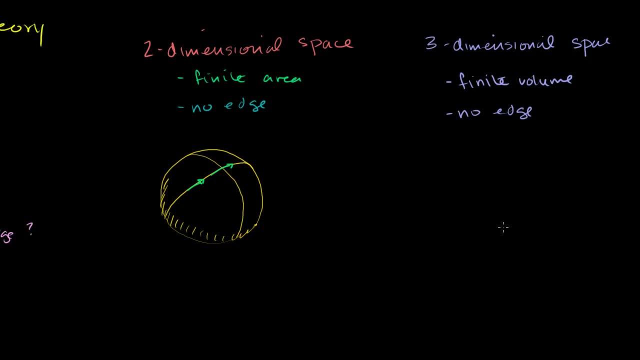 have to imagine it by analogy. Unless you have some type of a profound brain wired for more than three spatial dimensions, is a sphere. So let me make it clear: This is a two-dimensional surface. On the surface of the sphere, you can only move in two directions. 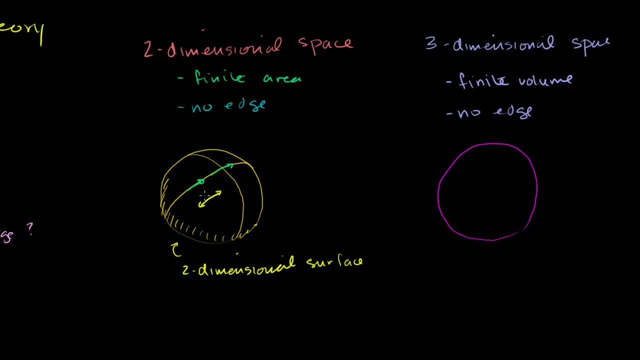 Two perpendicular directions. You could move like that or you could move like that. You could move left and right or you could move up and down. It's a two-dimensional surface of a three-dimensional sphere. So, if we take it by analogy, let's imagine: 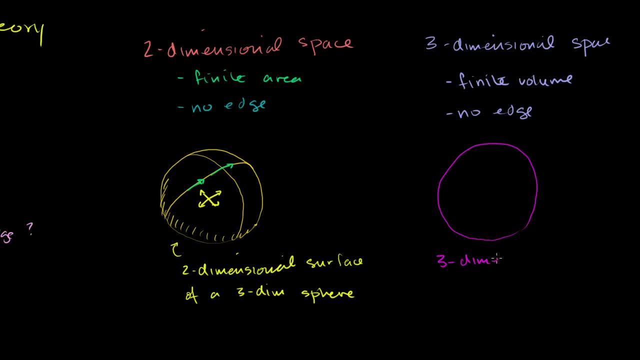 and it's hard to imagine a three-dimensional surface And you can do it mathematically. The math here is actually not that difficult. It's a three-dimensional surface of a four-dimensional sphere, Of a four-dimensional sphere, Of a four-dimensional sphere. 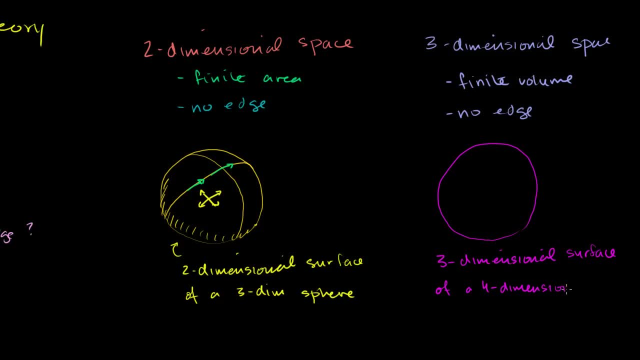 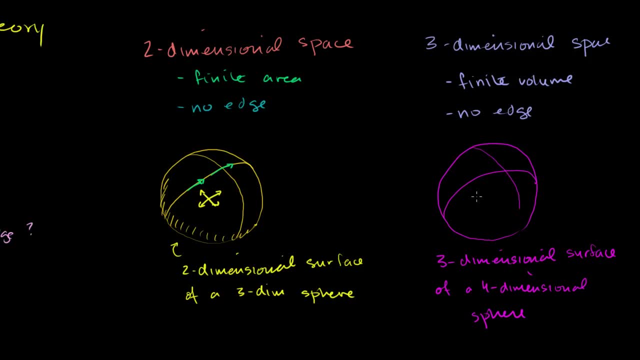 It's the same thing. And if you imagine that- and I'm not saying that this is actually the shape of the universe- We don't know the actual shape, but we do know that it does have a slight curvature. We don't know the actual shape, but a sphere is the simplest. 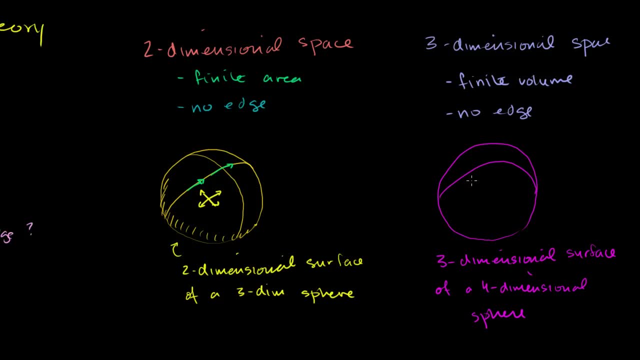 There's other ones we could do. A toroid would also fit the bill of having a finite volume With no edge. And another thing I want to make it clear: We actually don't even know whether it has just a finite volume. 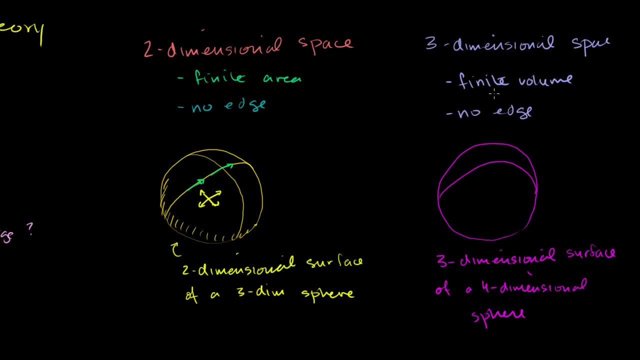 That's still an open question, But what I want to do is show you that it can have a finite volume and also have no edge, And most people believe, and I want to say believe here because we can just go based on evidence and all of that. 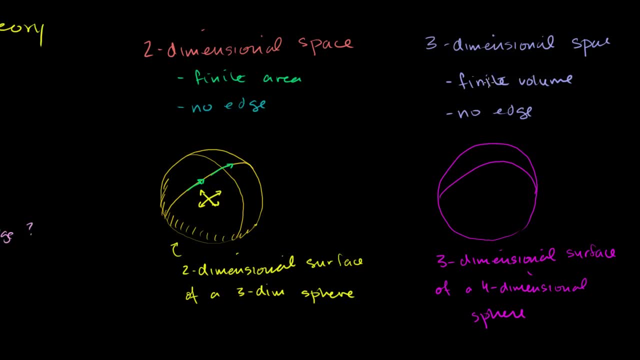 that we are talking about something with a finite volume, Especially when you talk about the Big Bang theory, That kind of, on some dimension implies a finite volume. Although it could be a super large, unfathomably large volume, it is finite. 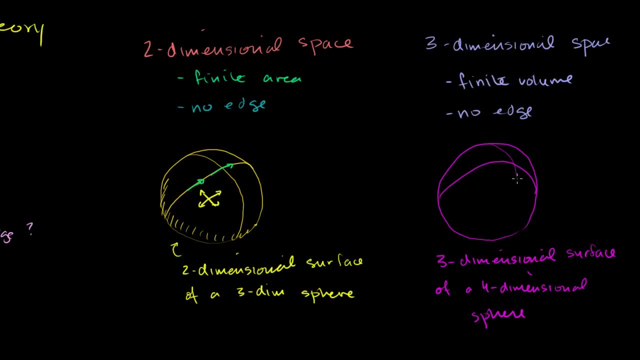 Now, if you have this, let's imagine this sphere Once again. if you're on this surface of this four dimensional sphere- I obviously cannot draw a four dimensional sphere, but if you're on the surface of this four dimensional sphere, if you go in any direction- 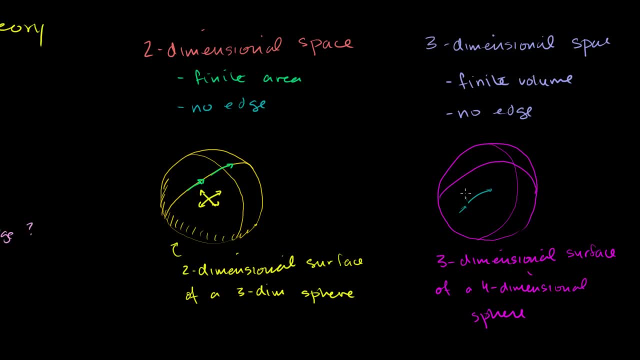 you'll come back out and come back to where you started. If you go that way, you'll come back around here. Now the universe is super huge, So even light- maybe light itself- would take an unbelievable amount of time to traverse it. 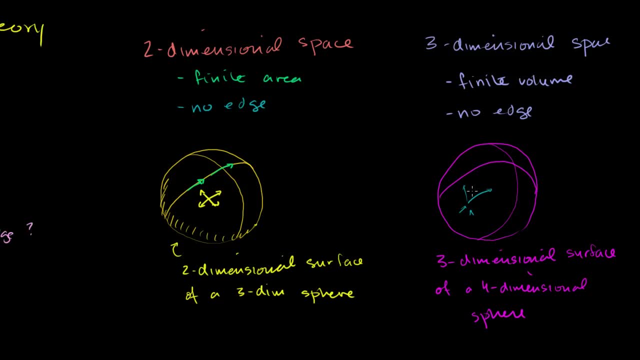 And if this sphere itself is expanding, it might be expanding so fast that light might not ever be able to come back around it. But in theory, if something were fast enough, if something were to keep going around, it could eventually go back to this point. 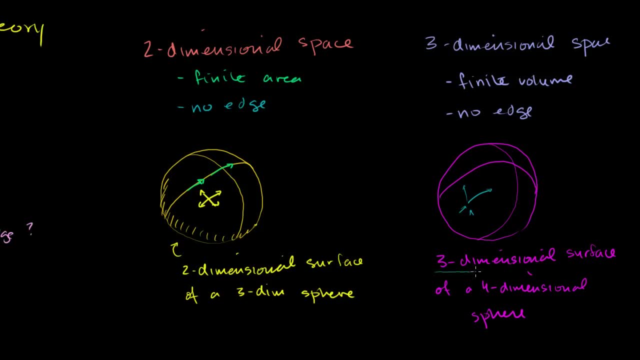 Now, when we talk about a three dimensional surface, it's a three dimensional surface of a four dimensional sphere. that means that any of the three dimensions over here on the surface, I can only draw two. But that means, if this is true, if the universe is a three. 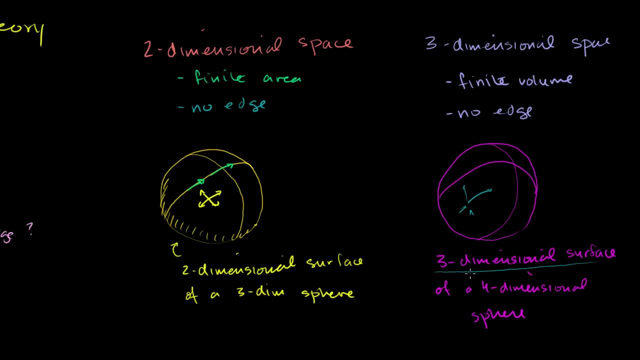 dimensional surface of a four dimensional sphere. that means that if you go up and you just keep going up, you'll eventually come back from the bottom. So if you keep going all the way up, you'll eventually come back to the point that you were. 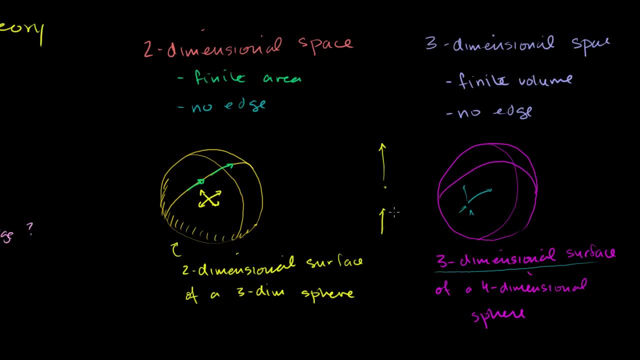 It might be an unbelievably large distance, but you'll eventually get back where you were. If you go to the right, you'll eventually come back All the way around to the point where you were. And if you were to go into the page. 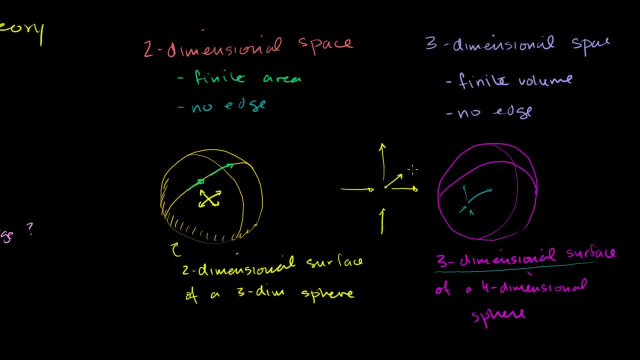 so if you were to go into the page- let me draw it that way- if you were to go into the page, you would eventually come back from above the page and come back to the point that you are. So that's what this implication would be. 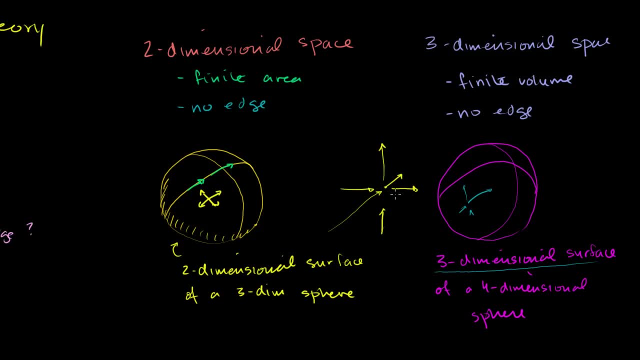 that you would eventually get back to where you are. So let's go back to the question of an expanding universe. An expanding universe that's not expanding into any other space, that is all of the space, but it's still expanding. Well, this is the model. 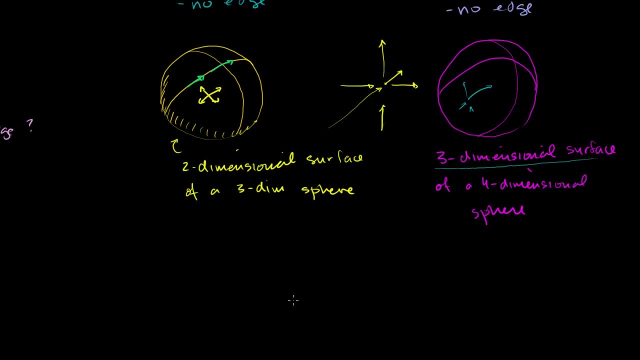 So you could imagine, Shortly after the Big Bang our four-dimensional sphere looked like this. Maybe it was a little small four-dimensional sphere. Maybe right at the Big Bang it was like this little, unbelievably small sphere. Then, a little bit later, it's this larger sphere.